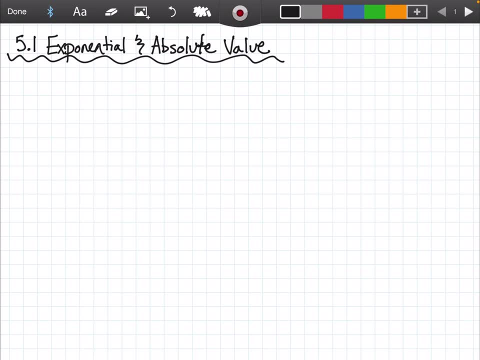 Welcome to Unit 5.. Very exciting stuff. Alright, let's talk about some exponentials and some absolute value. Basically, this unit is all about functions and systems of equations. So we're going to start with exponential, because that's something you've done before and we'll 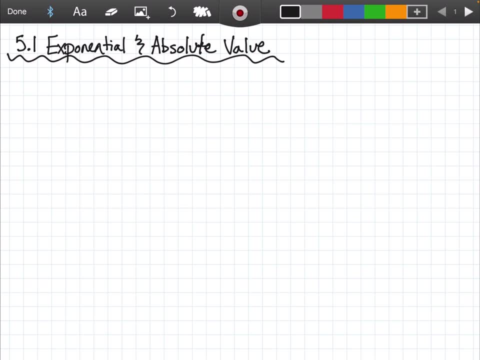 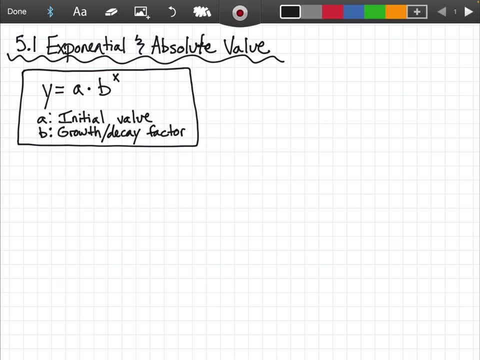 Talking about the rate of change of an exponential function, you know we have linear equations which have a constant rate of change, meaning you're adding or subtracting the same amount each time. Exponentials have a multiplicative rate of change, meaning we're multiplying. 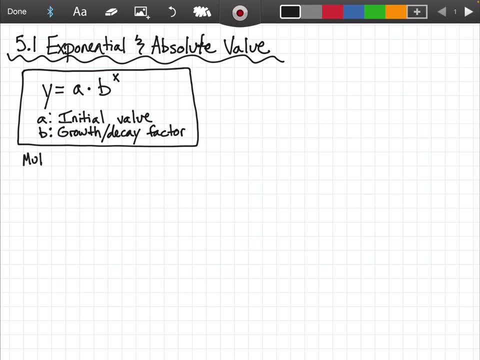 by the same thing every time, And that thing we're multiplying by each time is what we call the common ratio. So for some examples for you, let's say I have: f of x equals to the dx. Also just a reminder: f of x, that's just function notation. 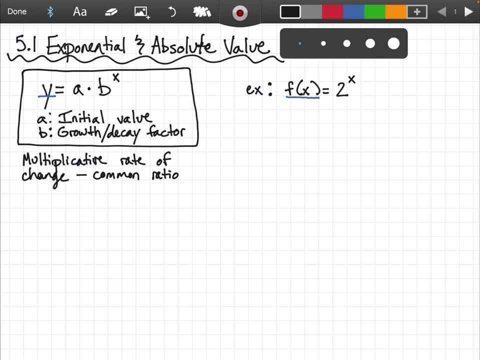 Same thing as saying y, And if I was to make myself a little table, let's see. alright, so I could just plug in my values here. First thing, I see Another way I could write this. It would be like one times two to the x, which tells me my initial value is one and my b. 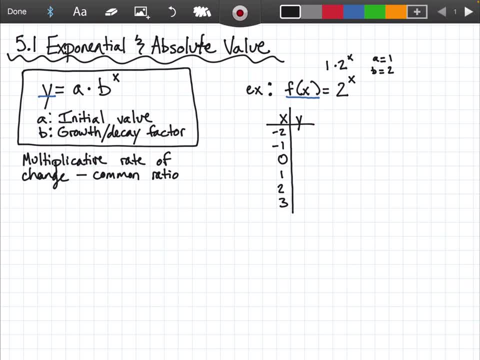 is two, And so we just need to see, like, how can we tell if this is growth or decay? Well, if I take a look and just start plugging in numbers, I'm going to start with two to the zero, because I know that anything to the zero, power is one. 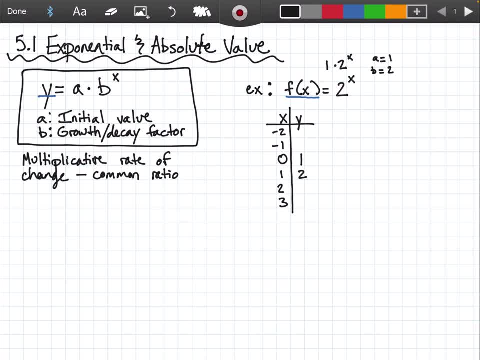 And now, if I plug in one, two to the first, power is two. If I plug in two, Two squared Two squared is four. If I plug in three, two cubed is eight. You see how I am multiplying by two every time as I go down the table. 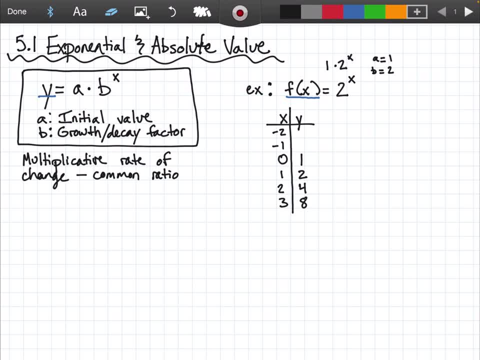 Well, that means if I were to go back up the table, I'm dividing by two every time, So I'd get a one half and a one fourth, which comes in with negative exponents. If you remember, two to the negative. two is like one over two squared, which becomes one. 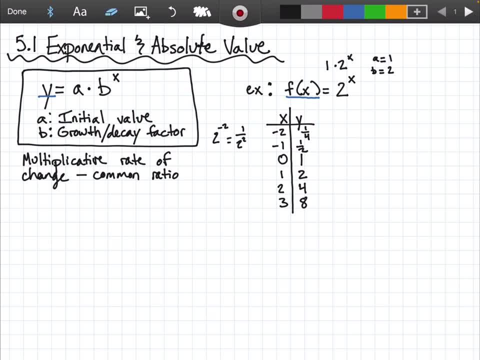 fourth, And so this one. I see, I see as I go down, we have growth. Let's look at another example. Let's say I have a different function. g of x equals one half all raised to the x power. Okay, 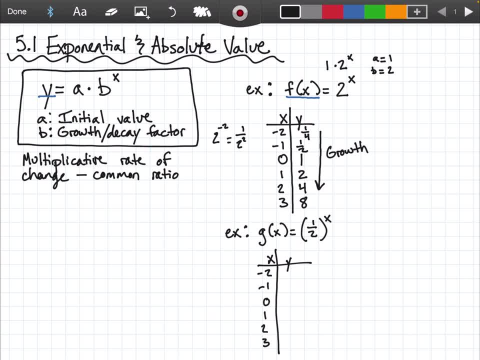 Okay, Okay, Okay. Let's go check this out. You can see this is about twice the same. Yup there. So we are having 0 again, because anything to the zero power I know is one That follows, because another way that we could write this would be like one times one half. 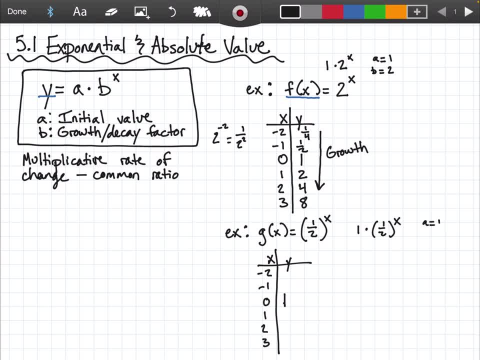 to the x. So my initial value is one. My growth slash decay factor is one half, And so one to the one half. power is one half. One half squared gives me one fourth, And one half cubed gives me one eighth. So you see how, as I go down the table, I'm dividing by 2, which means as I go up I can. 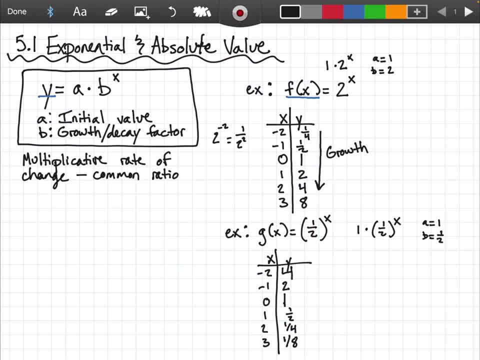 times by 2.. So this one is decay. So how do I know if I have growth or decay? It's all about the b-value or whatever your exponent is attached to. If it's bigger than 1, then it's growing. 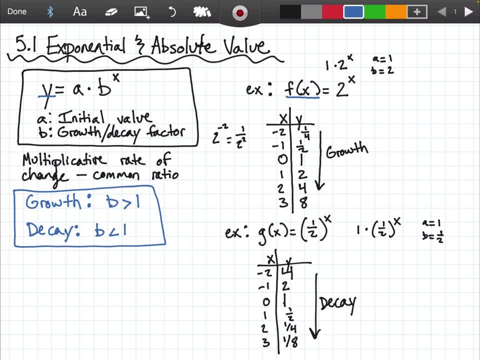 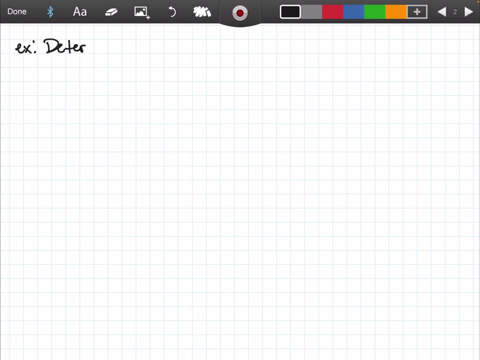 If it's less than 1,, it's decaying. If it's 1,, then that's just multiplying the initial value by 1 every time, And so that would actually not be good. It wouldn't be changing at all. So, for example, we're going to determine the initial value and the growth or decay. 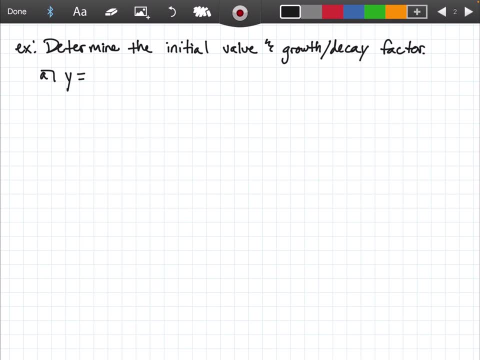 factor. Okay, So, for example A, my initial value is going to be 60, because that's what's out front of what's attached to the exponent And I can see this is growth, Because it's bigger than 1, so my growth factor is 1.41.. 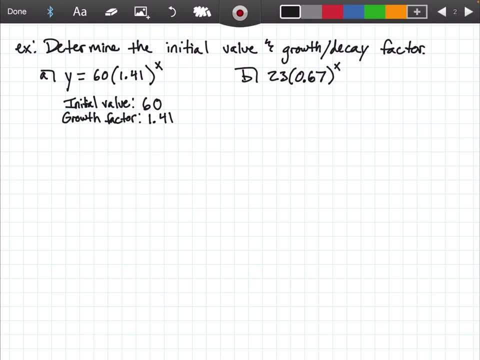 Another example: here I'm going to abbreviate initial value with IV: It's 23.. And this time I'm going to have a decay factor because it's less than 1.. Okay, My decay factor is 0.67.. 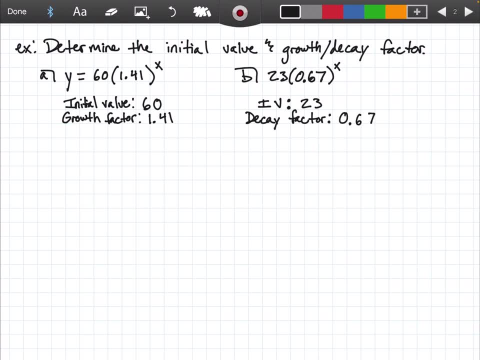 Cool. Well, we also need to talk about the growth decay rate. Okay, So I'm going to use a quantity here, Okay, Okay, the growth decay rate is the percentage change between – or I should say percent change – is the percent change between each output of the function. 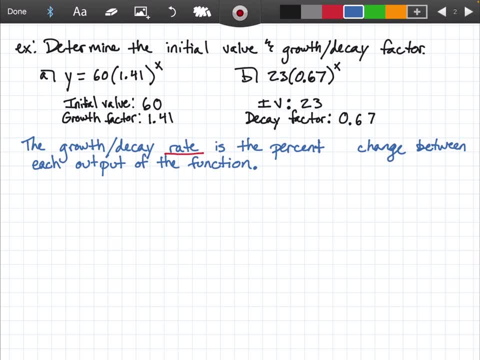 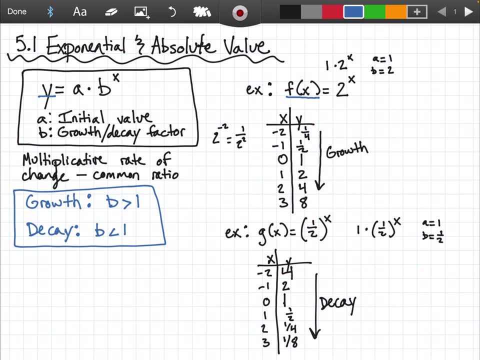 So meaning if I was to look back at our example of the table, let's look at our first example. You see how, from 1 to 2, it doubled. From 2 to 4, it doubled. From 4 to 8, it doubled. 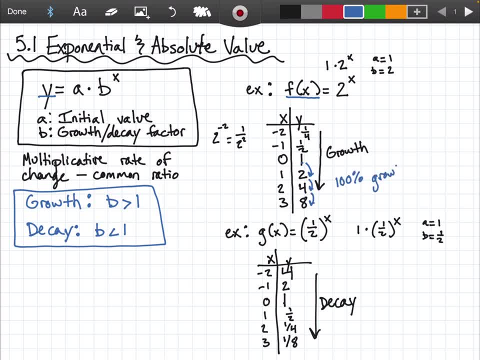 That is a 100% growth. every time if it doubles- Or here from 1 to 1.5,, it cut in half, cut in half, cut in half, which was a 50% decay. And so how do you think I got that? 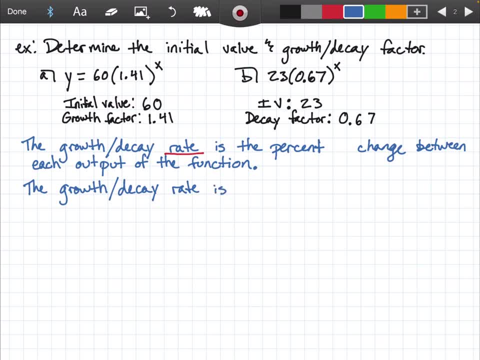 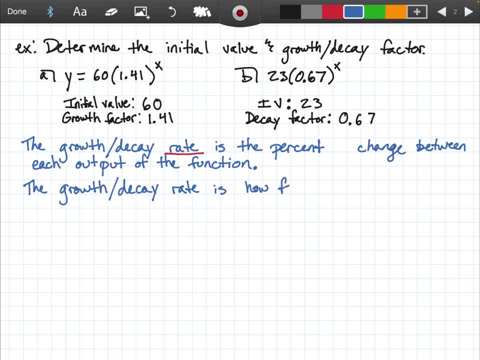 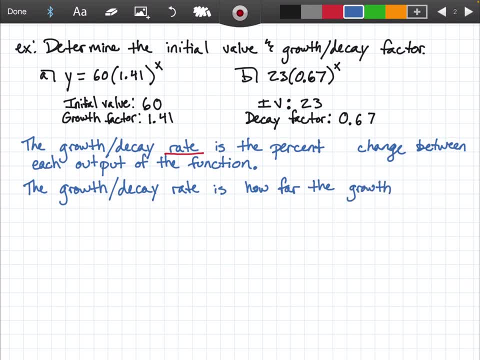 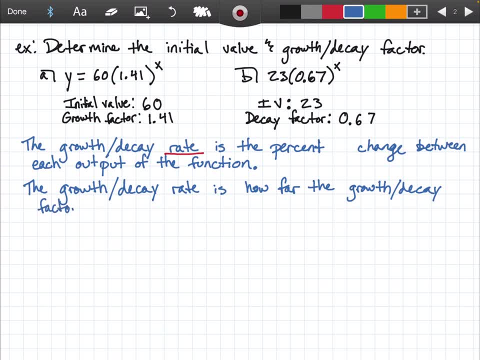 I think I got that from 1 to 4.. I think I got that from 1 to 4.. I think I got that from 1 to 4.. Alright, so we find the growth decay rate by how far the factor is from 1.. 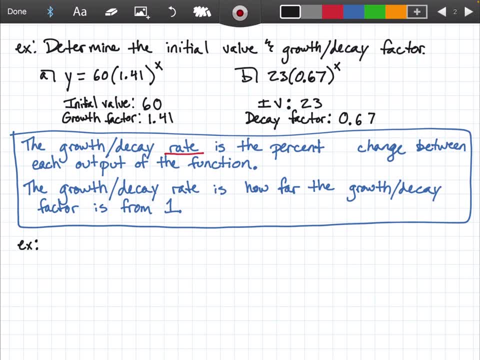 So, for example – So, for example, my initial value is going to be 5.. I know this is growth, because it's bigger than 1, and my growth factor is 1.47.. My growth rate is: how far is that factor away from 1.. 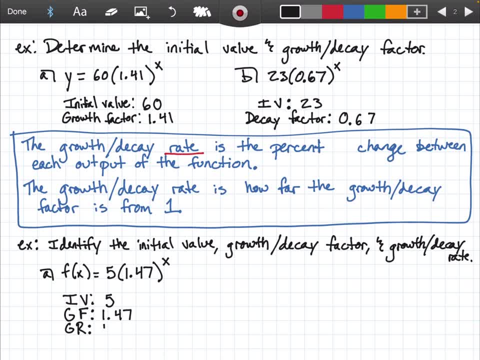 So that would be 0.47,, which is a 47% growth rate. Okay, I could also have something like – Y equals 4 times 0.78 to the X, where my initial value is the 4. This time it's decay because it's less than 1.. 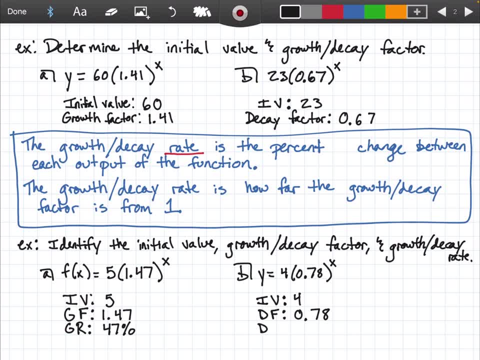 So my decay factor is 0.78.. My decay rate – How far is that away from 1?? Well, I can just do 1 minus that and we get 0.22.. 0.22, which means the decay rate is 22%. 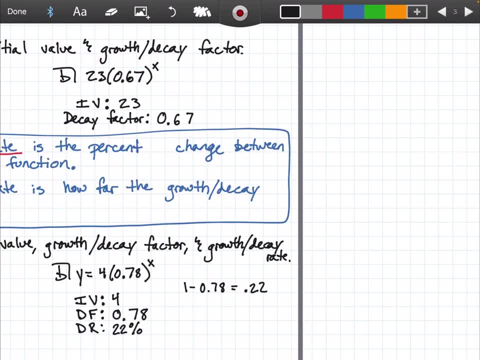 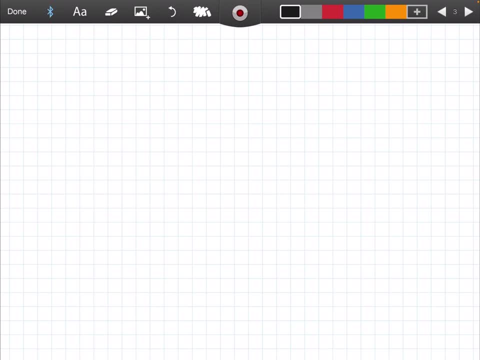 Okay, And last thing with this – Well, two more things. I'm going to do the same example, kind of example. I'm going to do the same example, kind of example. I'm going to do the same example, kind of example. 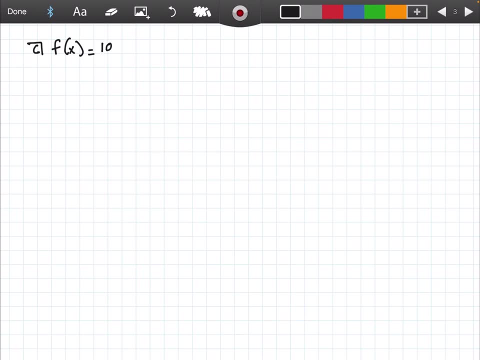 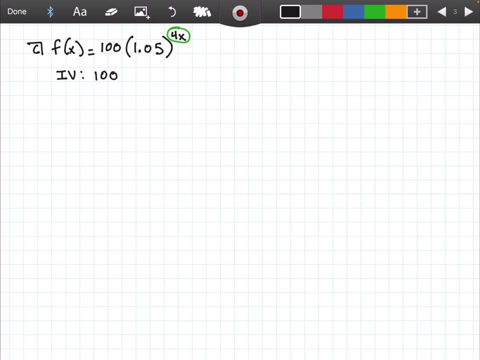 My initial value is still 100.. We're going to pull up properties of exponents for second. So we got 이렇게 một whippedσczyć Ig Beh� akl. divide by Z that must result in an half to the every step over here. 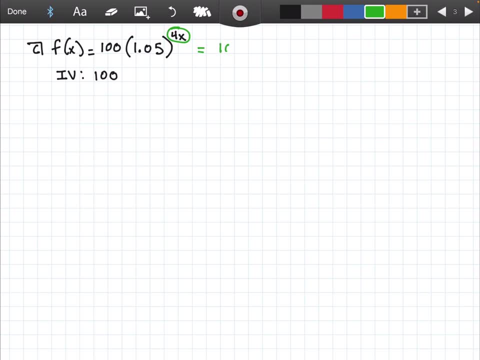 because this is the same as 100 times 1.05 to the 4th, all raised to the x. So it's like multiplying your exponents, And so in my calculator I can do 1.05 to the 4th and 1.22 to the x. 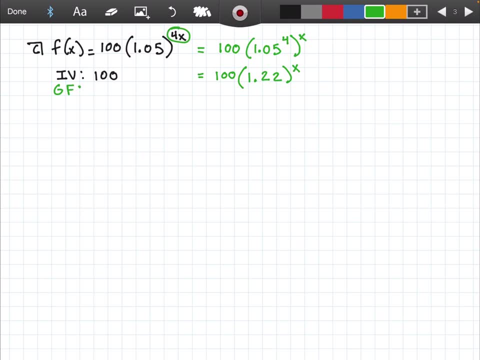 So that means really my growth factor is 1.22, which makes my growth rate 22%. Let's do another example like that, Something like this: Once again, I can pull up properties of exponents, because this would be equivalent to 0.68 to. 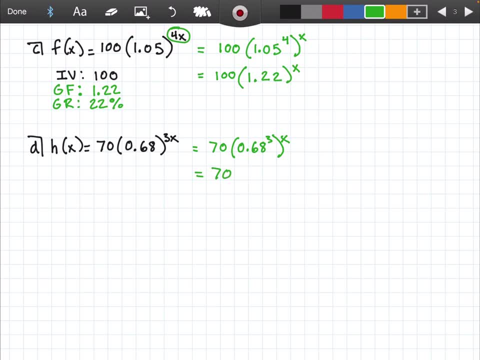 the 3rd, all to the x, which means this is really 70 times. let's see: 0.68 to the 3rd becomes 0.31.. Okay, Okay, So my initial value is 70.. This time my decay factor is 0.31, and my decay rate is 69%. 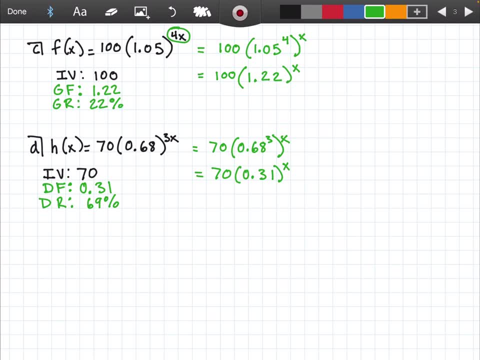 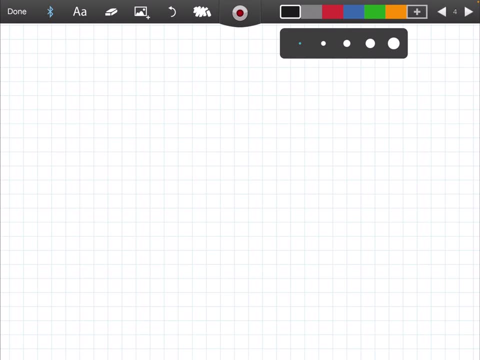 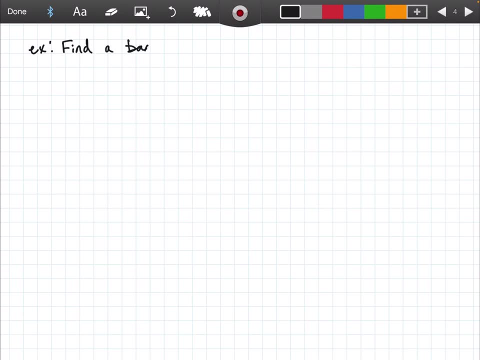 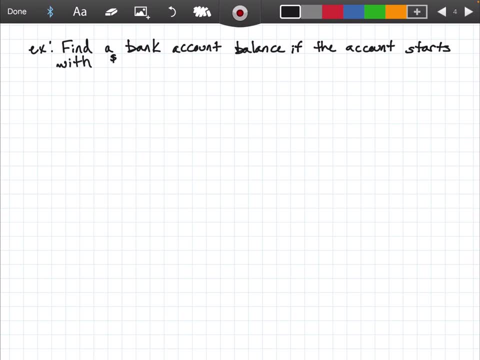 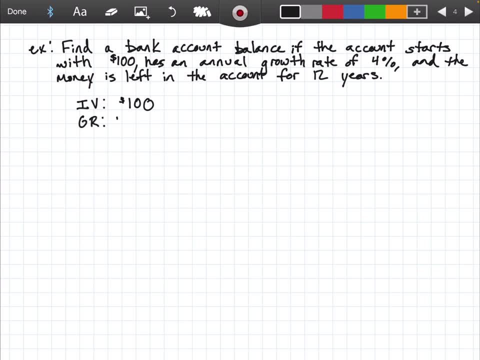 We know that the growth rate is 4%, which adds a decimal, So my initial value is 0.04.. Well, that means my growth factor is 1 plus that amount, so 1.04.. So my equation that I could put together is 100 times 1.04 to the x. 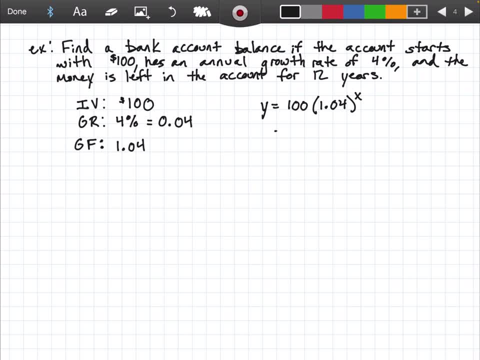 And x in this case is time, and so if we want to know how much is left in there after 12 years, we go 1.04, all to the x, And now we're going to type that in our calculator: 100 times 1.04 to the 12th, $160.10.. 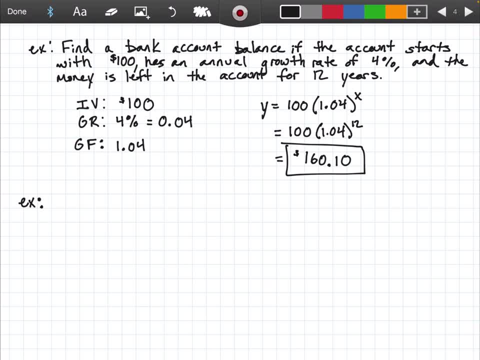 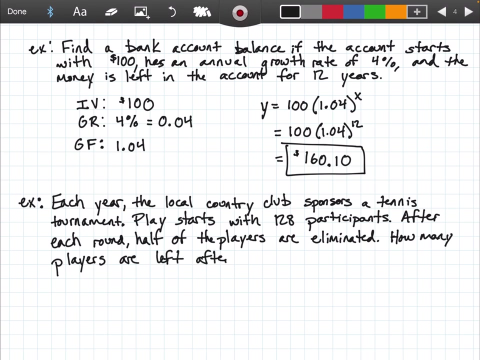 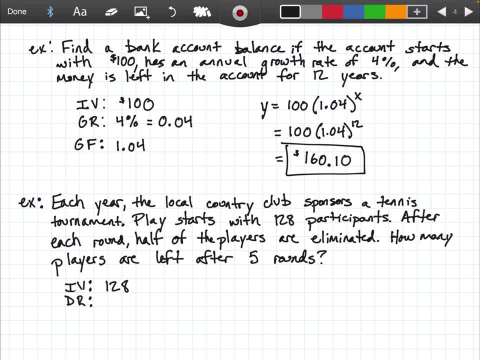 It's cutting in half every time. so cutting in half is 50% to 0.5.. So that means the decay factor is always 1 minus the decay rate. So in this case 1 minus 0.5 is still 0.5.. 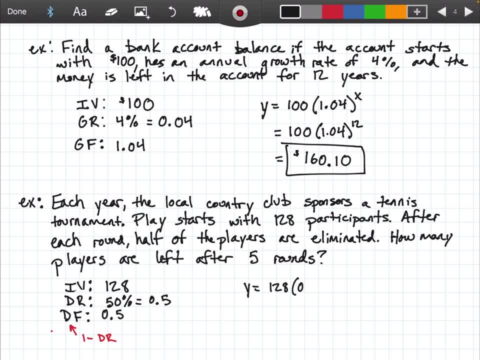 So it means my equation is 128 times 0.5.. So we're going to write 128 times 0.5 to the x. We want to know how many are left after 5 rounds. So 128 times 0.5 to the 5th. 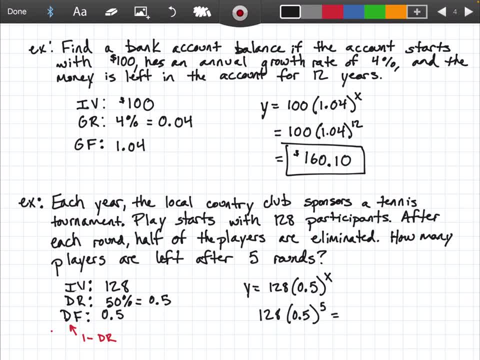 So after 5 rounds they get down to 4 players. These were the SOLT and they won. that was a way to sum this equation up, and I'm going to stop here because it was pretty hard and there's a lot more to go on with our tests. Thank you so much. Can κιver speak?